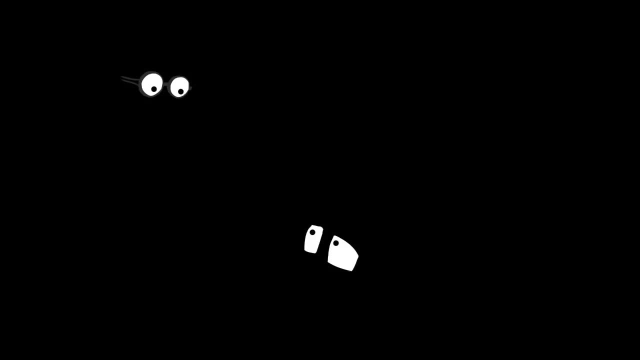 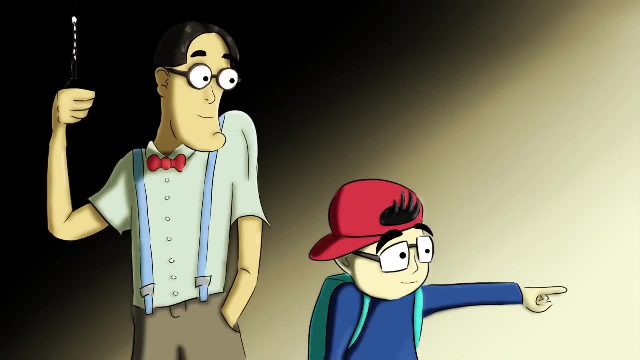 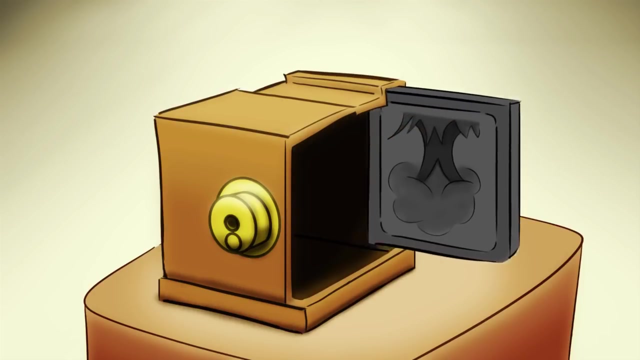 It sure is very dark in here. Well, that's because the camera is a light-proof box. It's built to capture light. Wow, What's that? That is a daguerreotype camera Developed from the camera obscura. it captures images on a silver-coated copper plate. 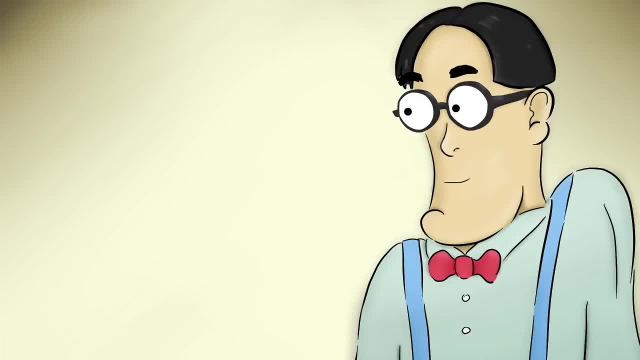 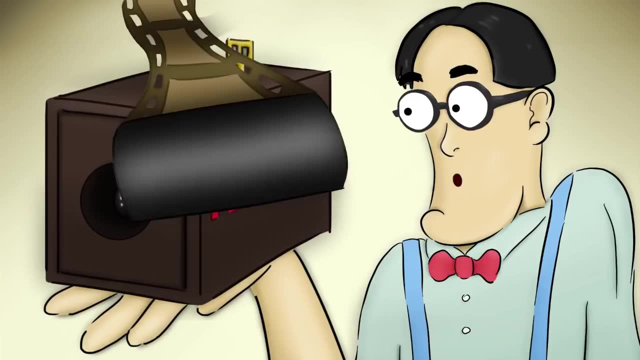 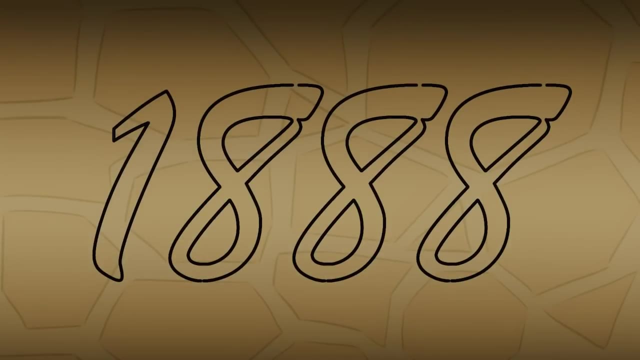 It was developed in 1839.. However, this is the first photographic film camera and it was invented by Kodak. It uses film strips containing light-sensitive silver halide crystals to capture images and was first introduced in 1888.. HmmHow does the camera work, though? 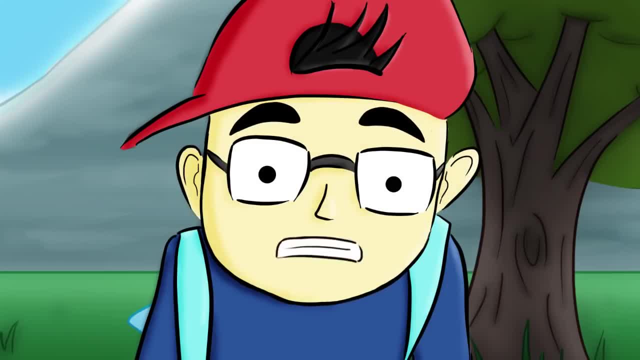 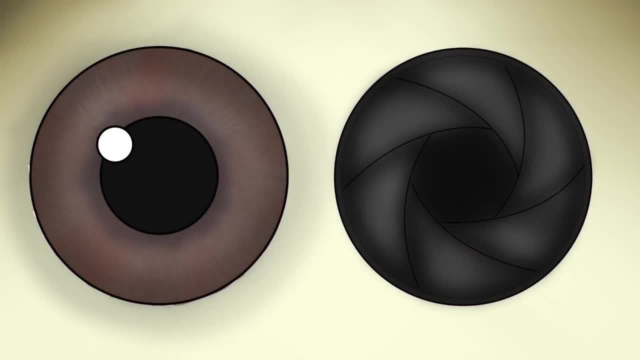 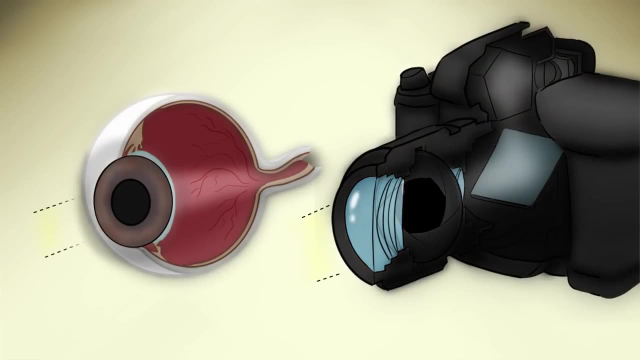 Well, a camera works the same way as your eyes, Alex. The diaphragm of the camera is like the iris of your eye and determines the amount of light entering the camera. Behind that there are lenses. Light bends when it travels at different speeds through different mediums, such as from air to glass. 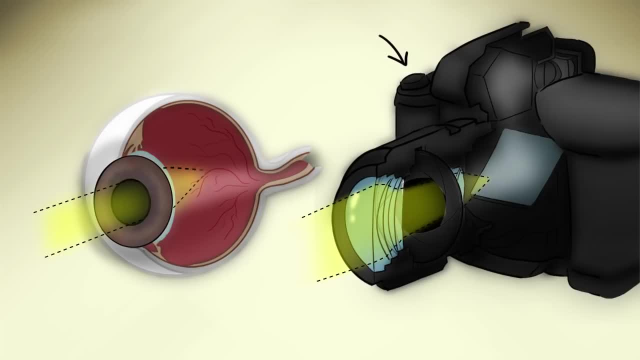 The light is then focused to a central point tournament-thrott in front. When you click on the shutter button, The movable mirror flips upward in the camera. The light stops when it reaches the film in the camera or the retina in your eye each. 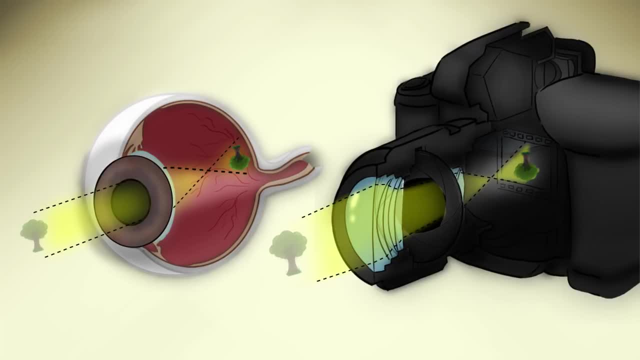 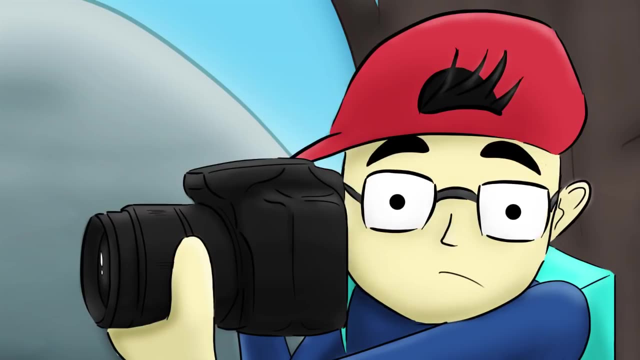 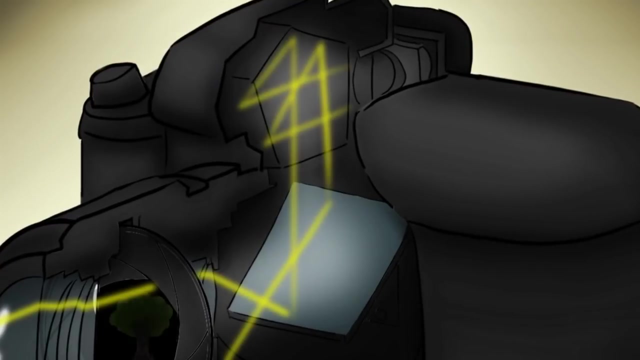 forms an inverted image. And why is the image upright when we see it in the camera? It's because there is another light path. When the shutter button is released, the movable mirror returns to its initial position. A pentaprism in the camera rotates the inverted image upright in the viewfinder. 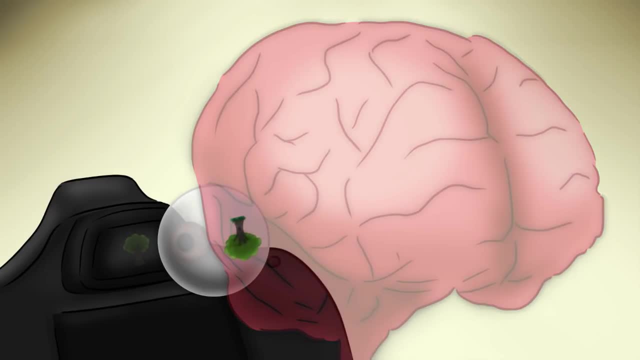 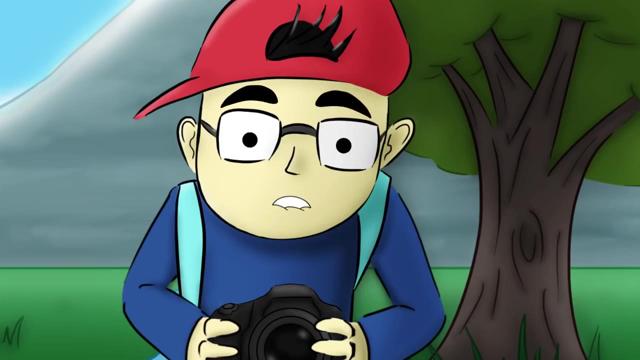 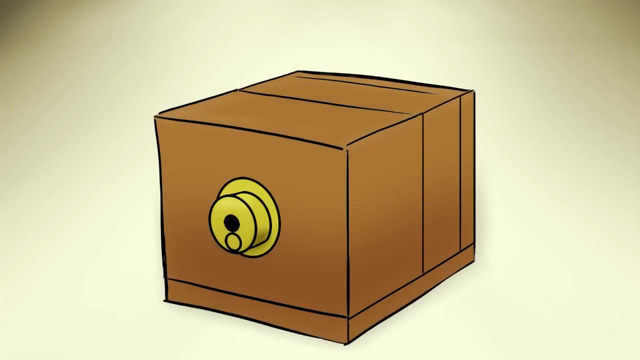 Even more amazing is when the image reaches the retina in our eyes, our brains process it to appear upright. Oh, so that's how the camera works. I have another question: What about digital cameras? Good question. As camera technology evolved, the way images were stored changed too. 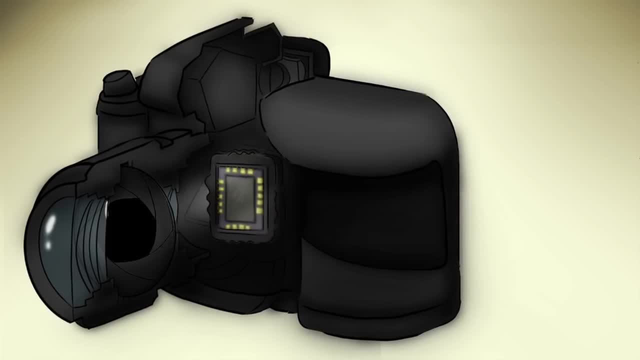 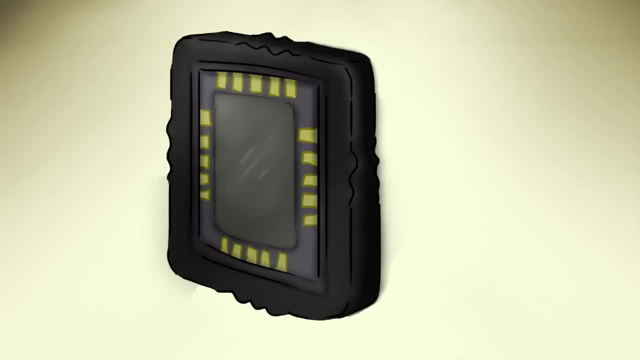 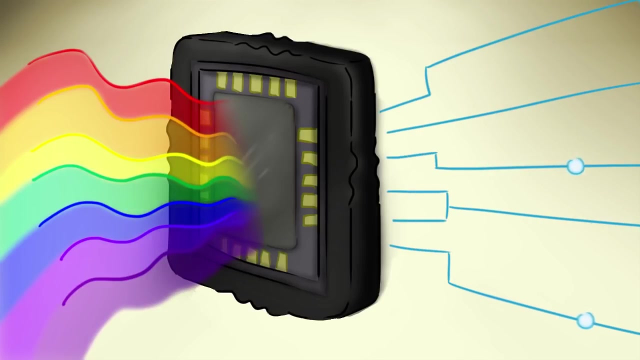 Photographic film strips were replaced with electronic film, giving birth to the digital camera era. Instead of using chemicals to react with light to form permanent patterns, electronic film picks up colors on a light-reactive surface and converts them into electric signals. These electric signals can then be translated by a computer into an image that can be displayed.